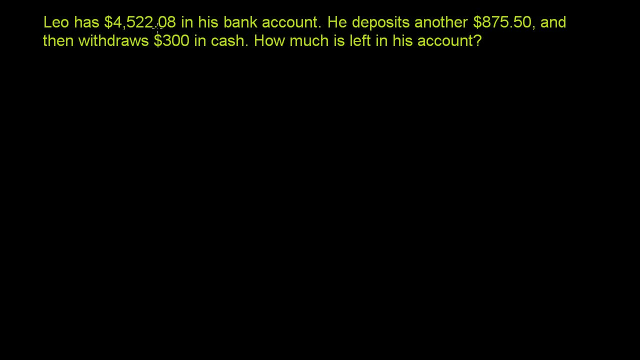 Leo has $4,522.08 in his bank account. He deposits another $875.50 and then withdraws $300 in cash. How much is left in his account? So he's starting with $4,522.08.. Let's write that down. 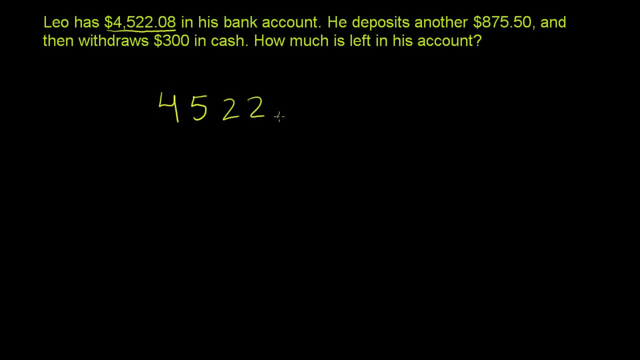 $4,522.08.. And then he deposits or he adds another $875.50.. So he's going to add $875.50.. When you deposit into an account, you're putting something into the account or you're adding to the account. 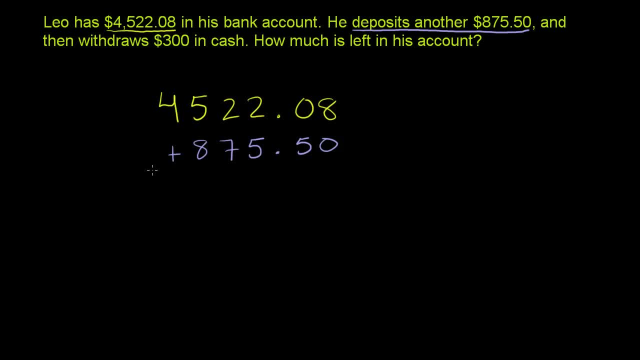 So after he adds that $875.50,, what does he have? So we go back to the penny spot, or we could view that as the hundredths. A penny is one hundredth of a dollar, $875.50.. Let me switch colors. 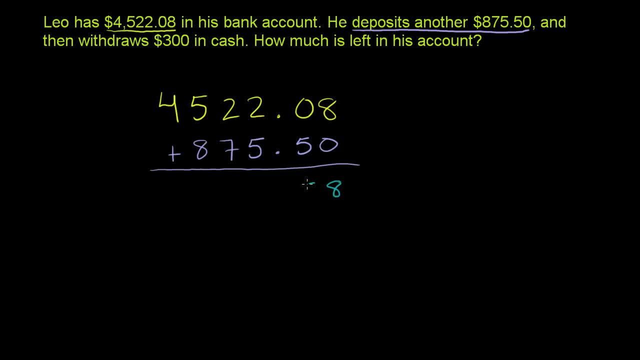 We have: 8 plus 0 is 8.. 0 plus 5 is 5.. Have the decimal right there. 2 plus 5 is 7.. 2 plus 7 is 9.. 5 plus 8 is 13.. 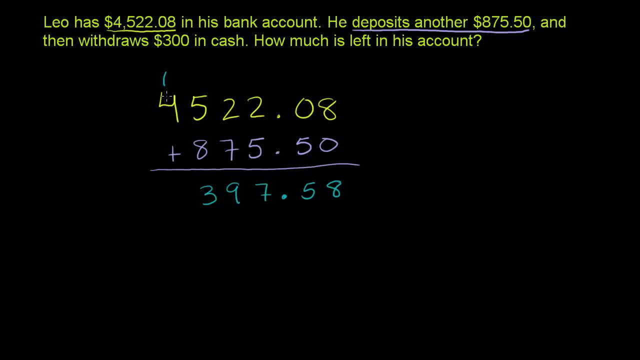 Put the 3 down here and regroup the 1 or carry the 1.. 1 plus 4 is 5.. So after the $875.50 deposit he has $5,397.58.. Then he withdraws. He withdraws $300 in cash or he takes out $300. 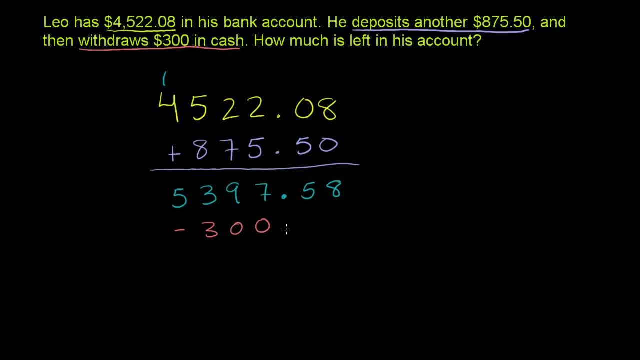 So we'll have to subtract that. So then he withdraws $300. And I just added some trailing zeros after the decimal. $300 is the same thing as $300.00. And then we subtract, And then we can subtract: 8 minus 0 is 8.. 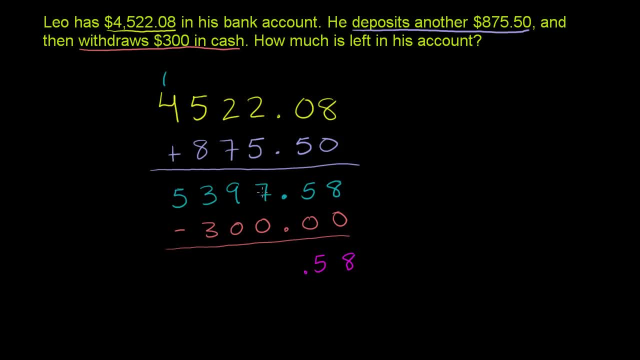 5 minus 0 is 8.. 5 minus 0 is 5.. We have our decimal right there. 7 minus 0 is 7.. 9 minus 0 is 9.. 3 minus 3 is 0.. 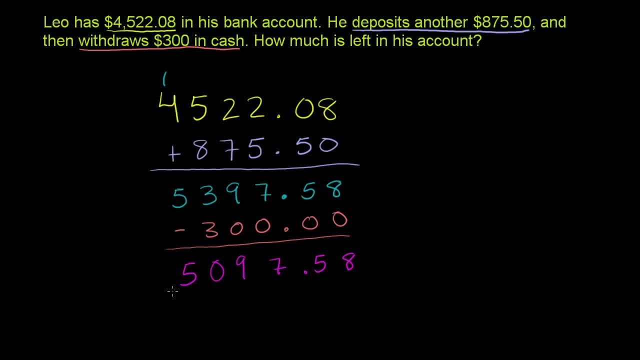 And then 5 minus nothing here is 5.. So he's left with in his account $5,097.58..